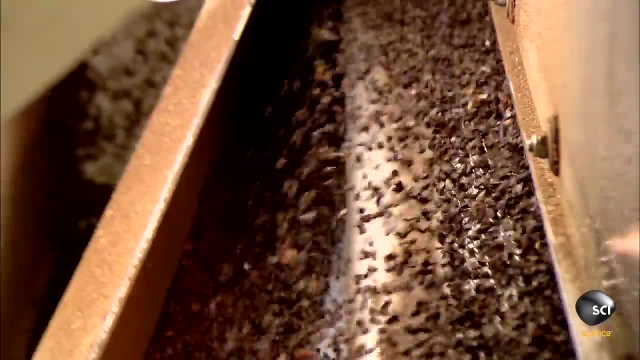 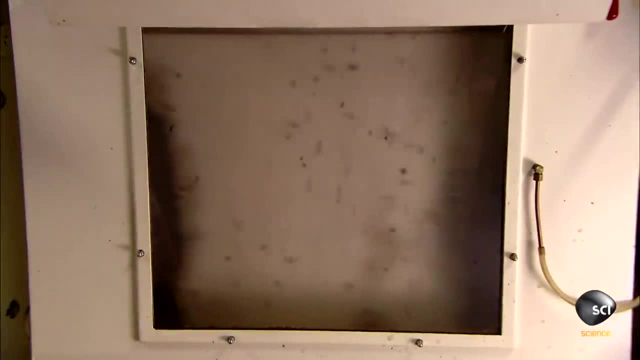 called a winnower. Inside, successive rakes drag the beans across screens, pulling off large pieces of shell. Then a vacuum sucks away the remaining smaller pieces. Removing the shell exposes the inside of the cocoa bean, which is called the nib. 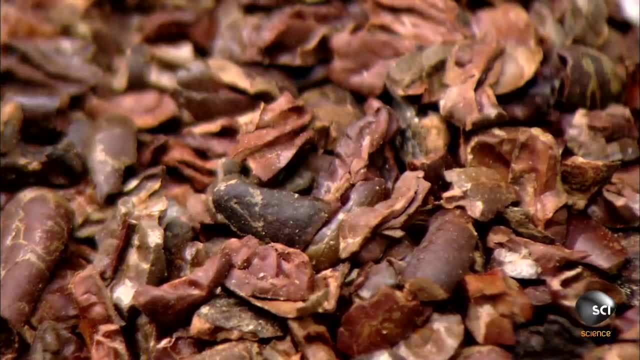 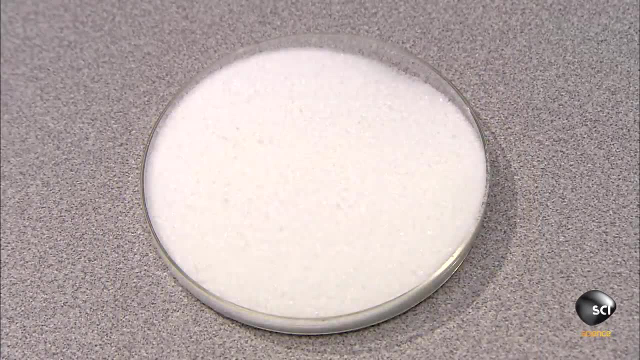 The factory will roast the nibs to develop their flavor. 50 plus percent of the nib is fat, which is cocoa butter. To make chocolate, they'll combine processed nibs, cocoa butter and sugar, along with milk powder, if they're making milk chocolate First. 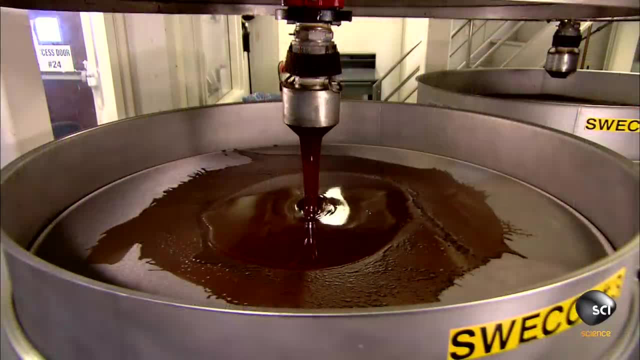 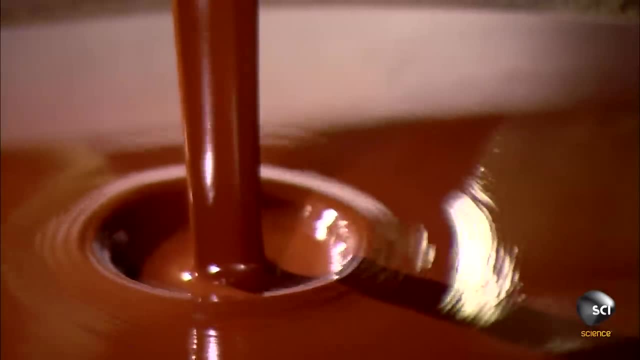 the factory will make chocolate. The factory will make chocolate. The factory will make chocolate. The factory processes the nibs by grinding them. The heat and friction activate the cocoa butter, producing pure liquid chocolate called chocolate liquor. The factory extracts some of the cocoa. 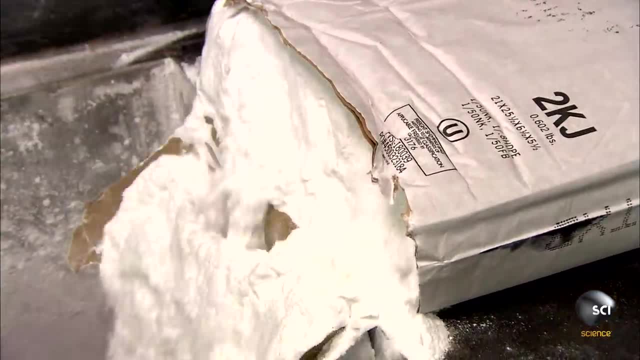 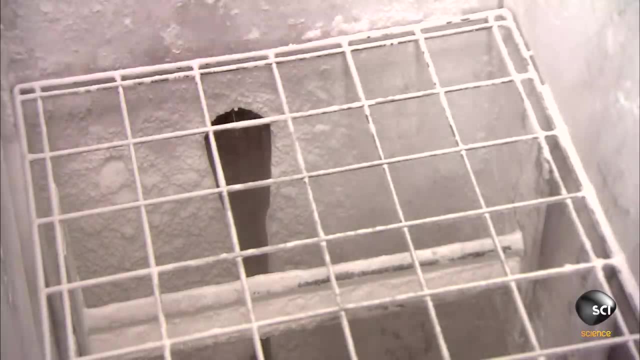 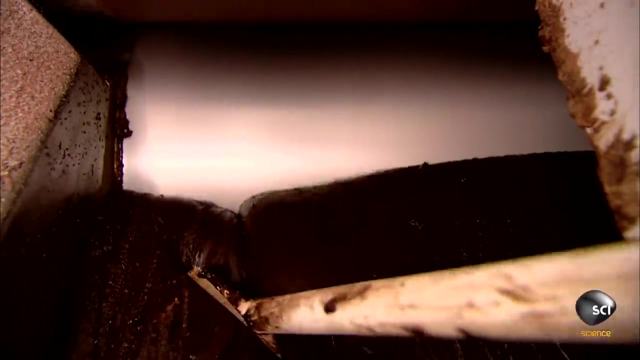 butter, to sell it separately as chocolate making ingredient and to use for in-house chocolate production along with other ingredients in various proportions. The dark chocolate recipe, for example, calls for more chocolate, liquor, sugar and cocoa butter, but no milk powder. The recipe for unsweetened chocolate contains no sugar. The mixer blends the ingredients to the 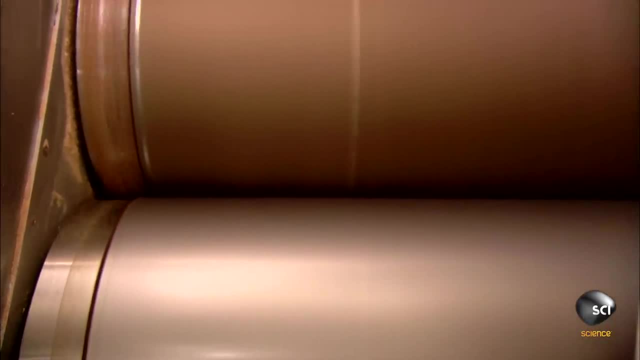 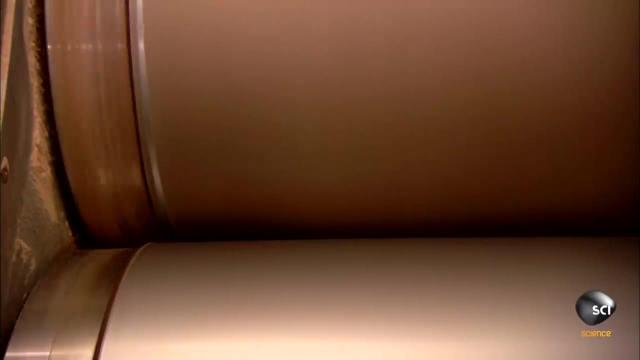 consistency of a very thick cake batter. The flavor is fine by this point, but the coarse texture needs to be smoothed out. So the chocolate moves to a refining machine, passing between a set of five rollers that reduce the particle size so much so that 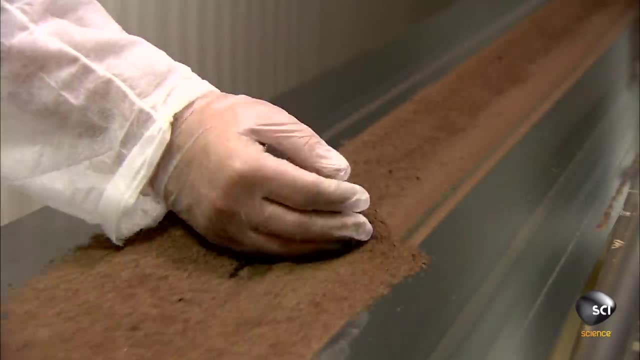 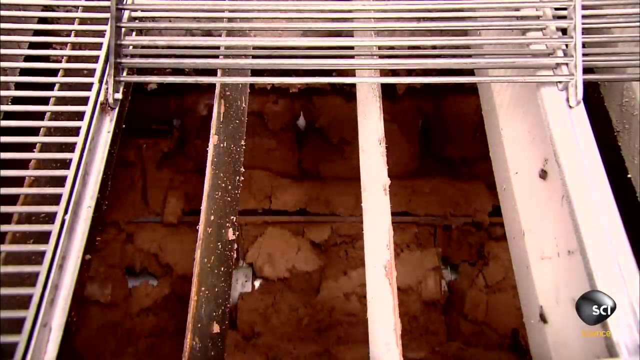 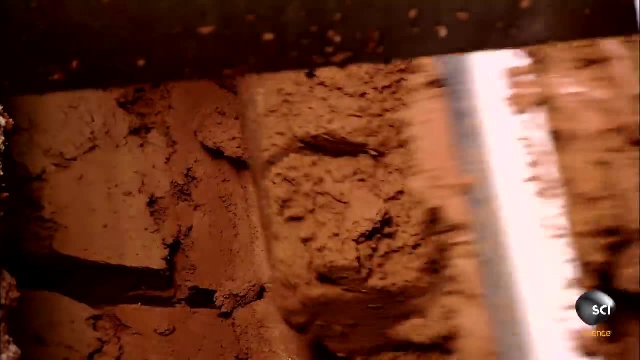 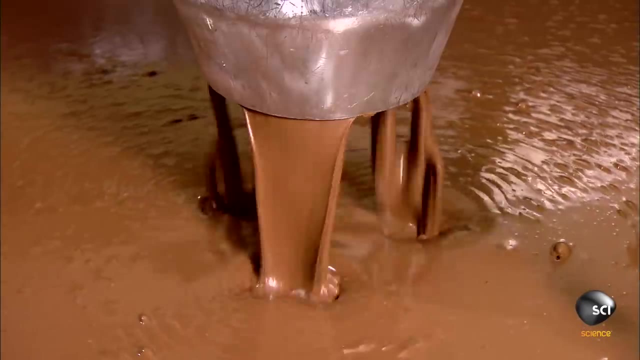 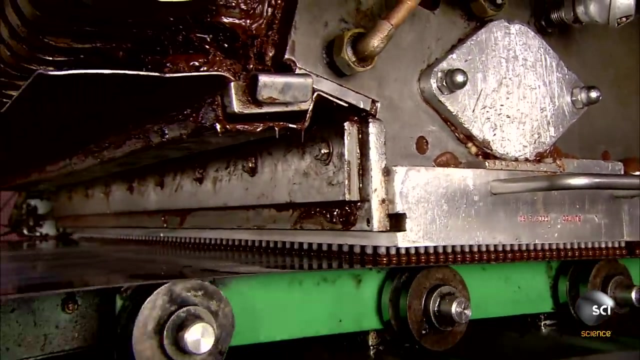 The friction and heat once again activate the cocoa butter, returning the powder to a liquid state. At this point they add more cocoa butter- enough to reduce the viscosity to the exact thickness they need- Just a bit, for example, if they're making chocolate chips, or much more if they're 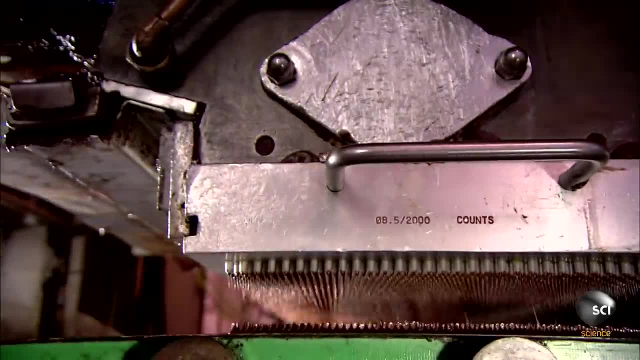 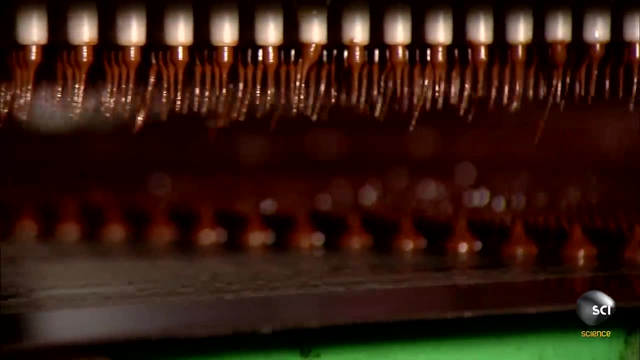 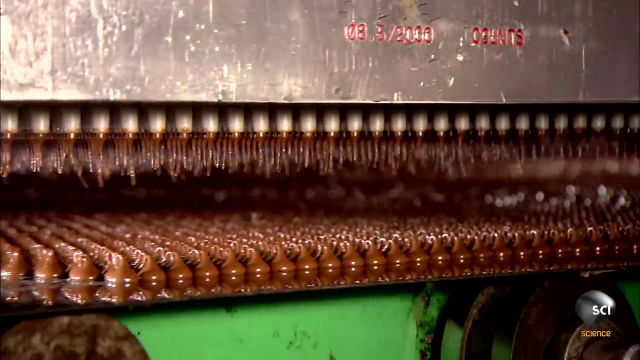 making a thin chocolate coating For chocolate chips. the conch feeds a machine called a drop filter. As the name implies, it deposits drops of chocolate onto a conveyor belt. The nozzle trays are interchangeable, so the machine can be set up to produce various sizes.